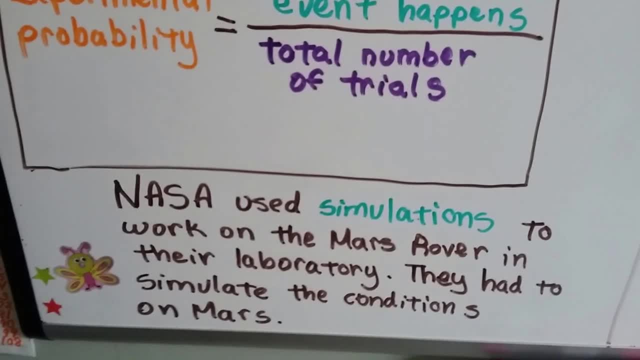 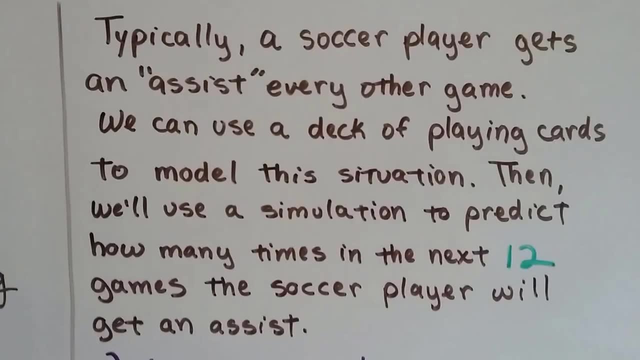 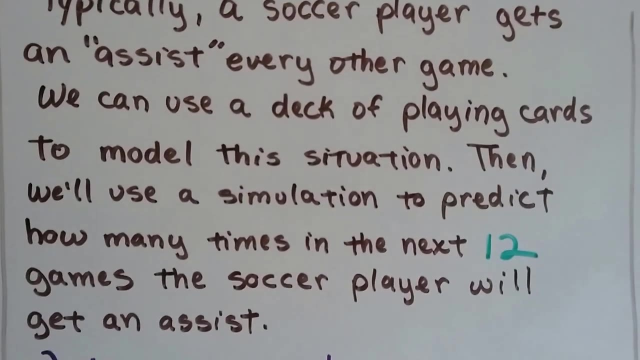 And then they designed the Mars rover according to those simulations. Okay, So it helps. when you do simulations in an experiment, Typically a soccer player gets an assist every other game. We can use a deck of playing cards to model this situation. Then we'll use a simulation to predict how many times in the next 12 games the soccer player will get an assist. 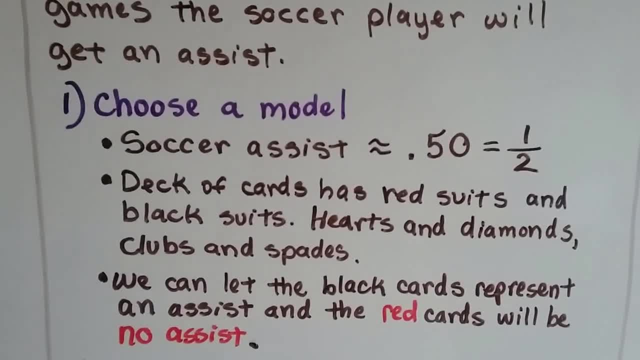 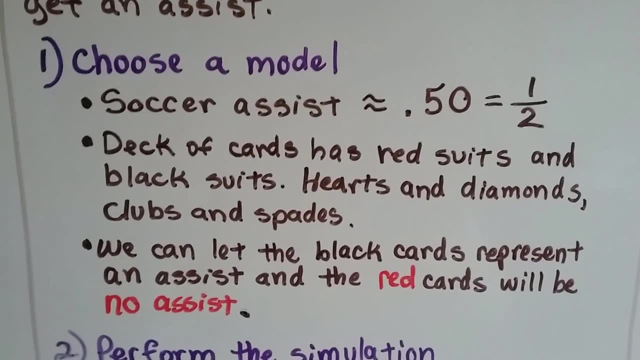 So we choose the model. That's the first thing, That's the soccer assist, And it happens approximately 50% of the time, or 0.50, which is half right. We can use a deck of cards because they have red suits and 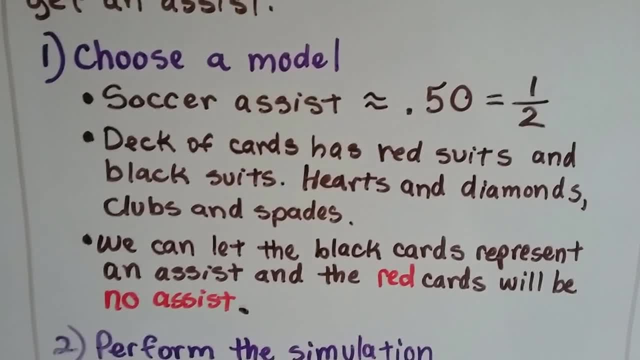 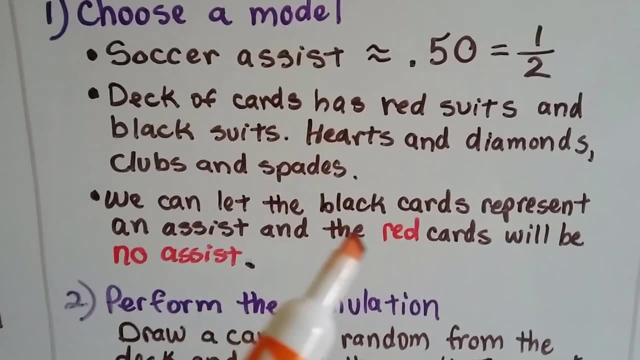 black suits, the hearts and diamonds versus the clubs and spades. That's 50-50, right. Like the soccer assists, We can let the black cards represent an assist when he gets help And the red cards will be no assist when there's no help. 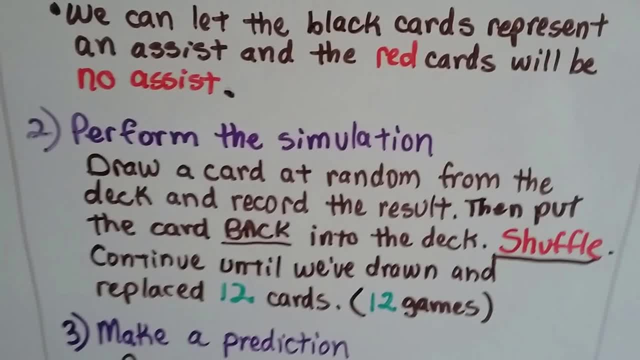 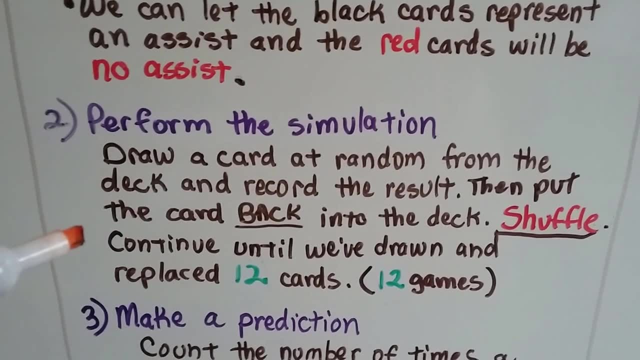 Okay, So we have to hope for a black card. Perform the simulation is the next step. We draw a card at random from the deck and we record the result. Then we put the card back into the deck, We shuffle it and then continue until we've drawn and replaced 12 cards. 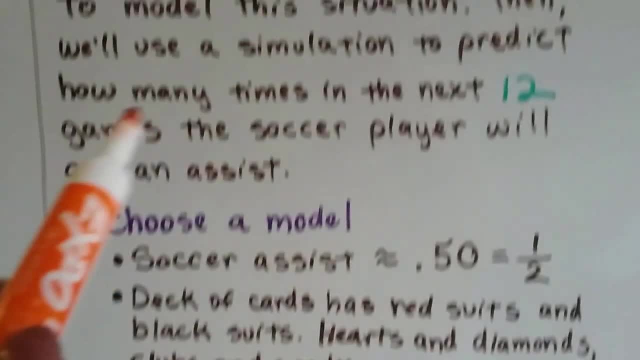 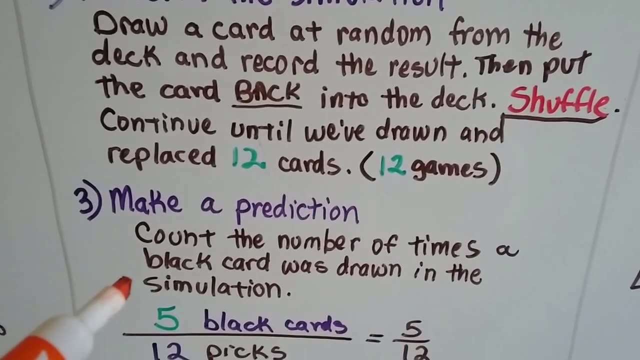 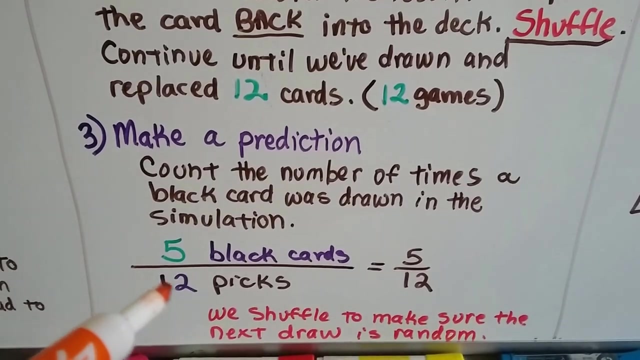 There's 12 games, See. So we want to do it for 12 cards. So we make a prediction, We count the number of times a black card was drawn in the simulation And if we picked five black cards out of 12 picks, that's five twelfths. 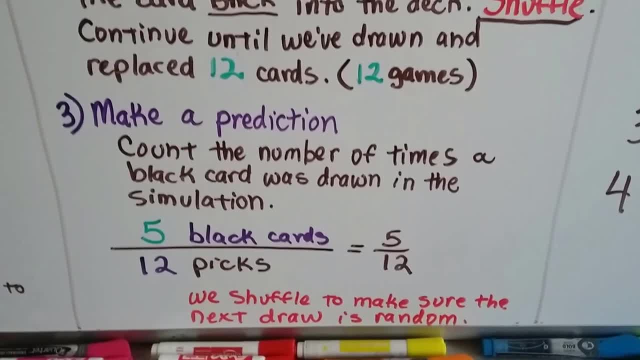 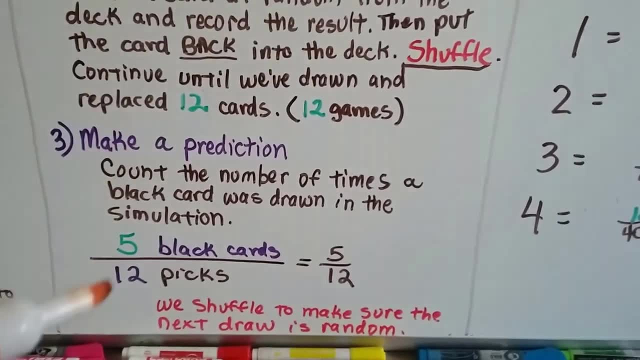 See, Now it's important that you shuffle the deck because you want to make sure that each draw that you do is random. If you kept putting them back in the simulation, you wouldn't get a draw. If you kept putting them back in the same spot, it wouldn't be as random. 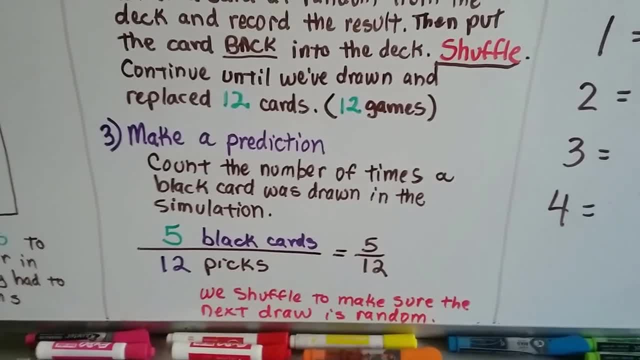 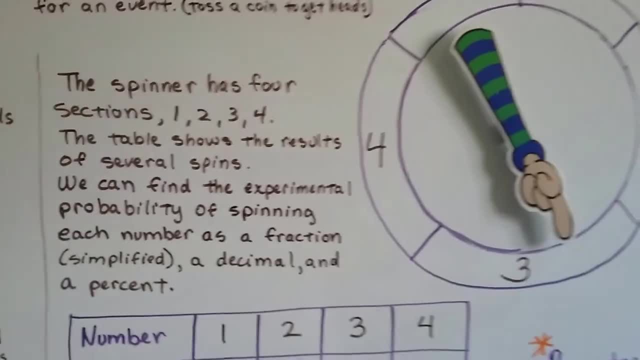 So shuffling them really makes sure you don't know what the next card is going to be See. All right, We want them to be random, We want it to be fair and unbiased, right? So here's our friend the spinner. 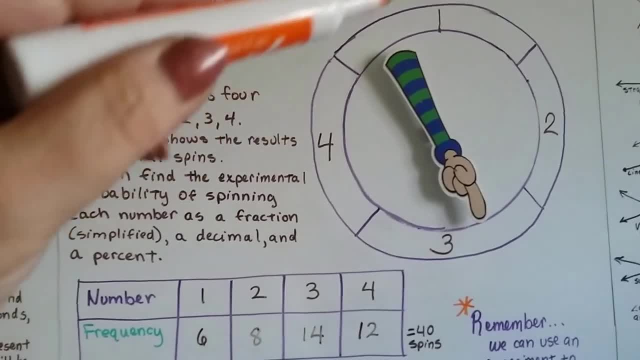 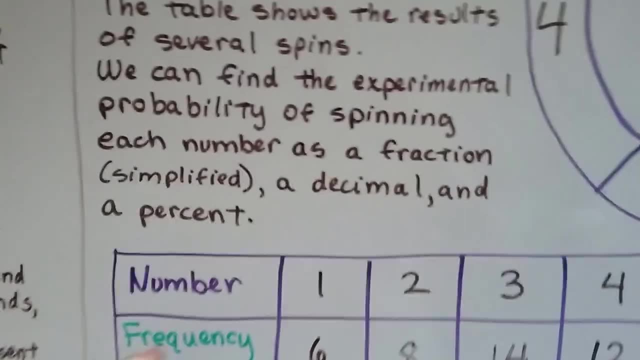 Remember last video? he had colors around him, So now he's got numbers 1,, 2,, 3,, 4.. So the spinner has four sections: a 1,, 2,, 3, and 4.. And this table right here shows the results of several spins. 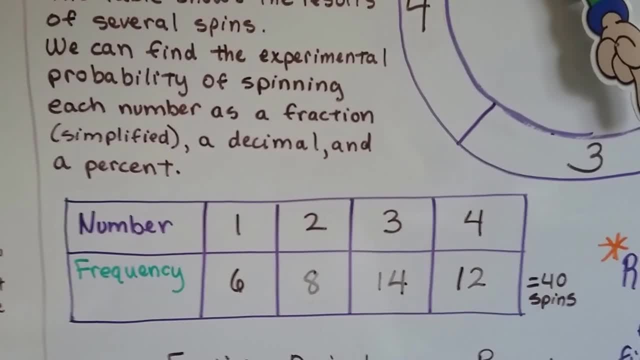 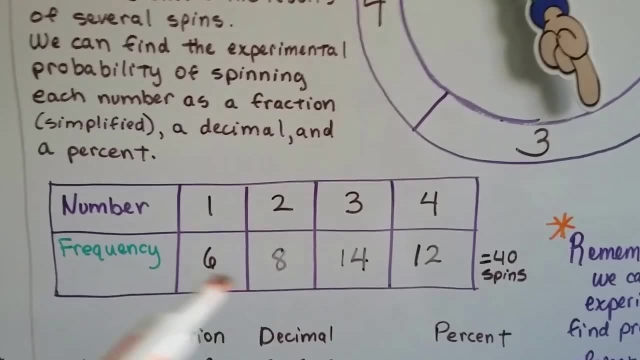 So we did 40 spins. We can find the experimental probability of spinning each number as a fraction, simplified of course, and a decimal and a percent. So if there was a total of 40 spins, that's going to be our denominator, okay. 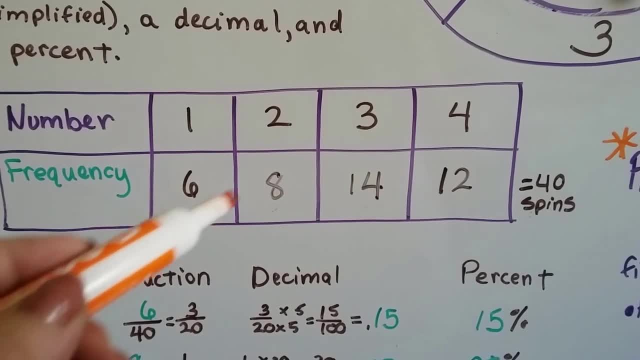 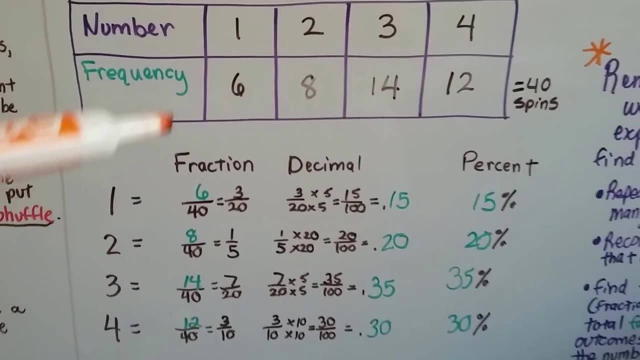 Here's the frequency: It landed on 1 six times And it landed on 2 eight times. It landed on the 3 14 times And it landed on the 4 12 times. So, as a fraction, it landed on the 1: 6 out of 40 spins. 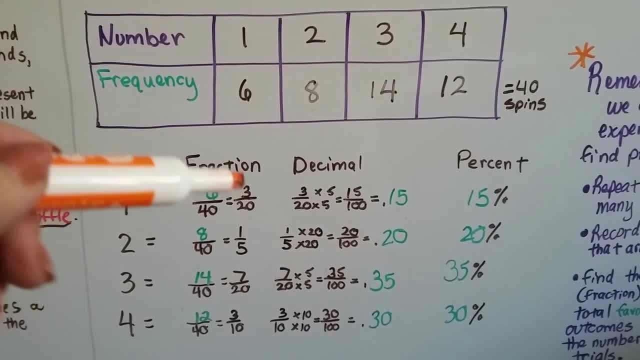 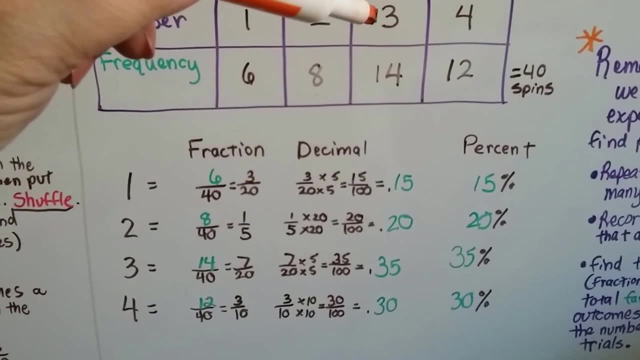 So it's 6 40ths. We reduce it to 3- 20ths. It landed on the 2, 8 out of 40 spins, So that's 8 over 40.. That's 1 fifth of the time. 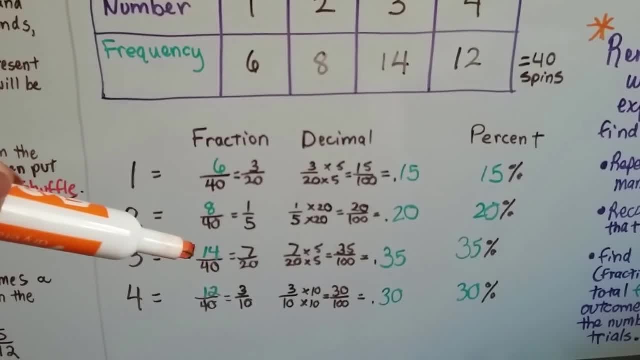 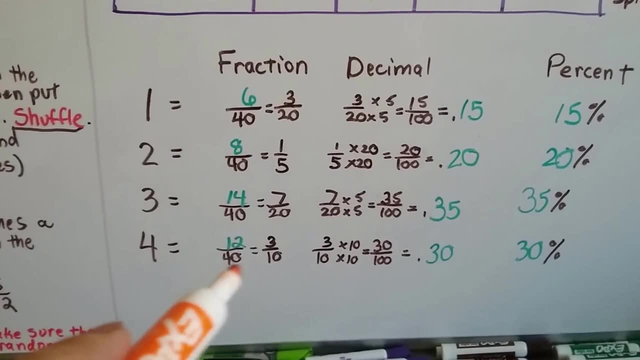 It landed on the 3, 14 out of 40 times. We reduce that to 7- 20ths. And it landed on the 4 12 times out of 40 spins. That's 12 over 40, or 3 tenths. 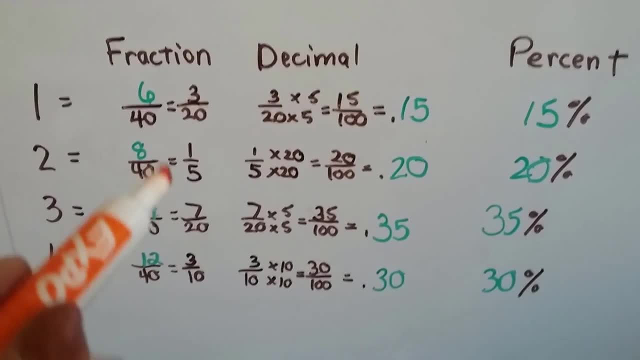 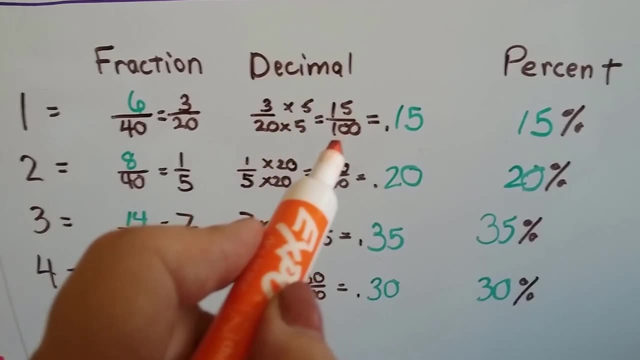 Now as a decimal. do you remember how to convert fractions to decimals? We look at the denominator. We're going to use the 3, 20ths, And what does the denominator need to become 100?? It needs to be multiplied by 5.. 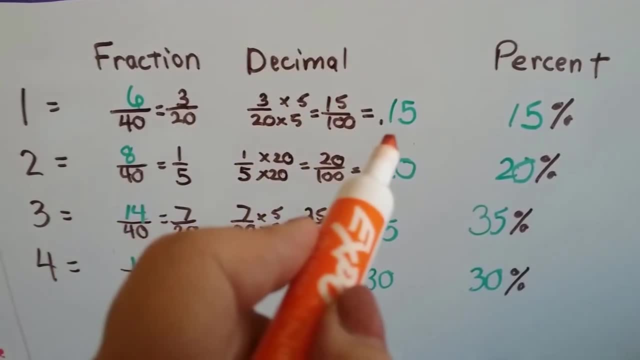 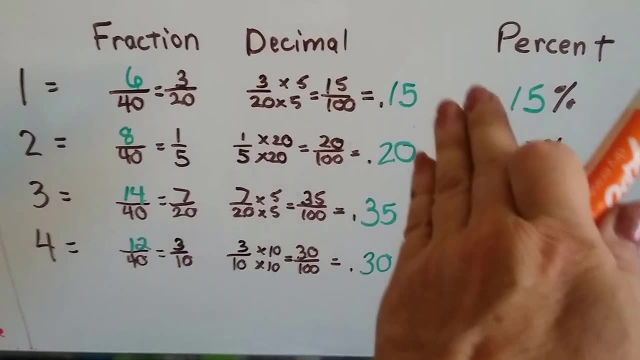 So that's what we do to the numerator. So it becomes 15 over 100, or 15 hundredths. 1 fifth becomes 20 hundredths or 2 tenths. right, Because we could take that 0 off if we wanted to. 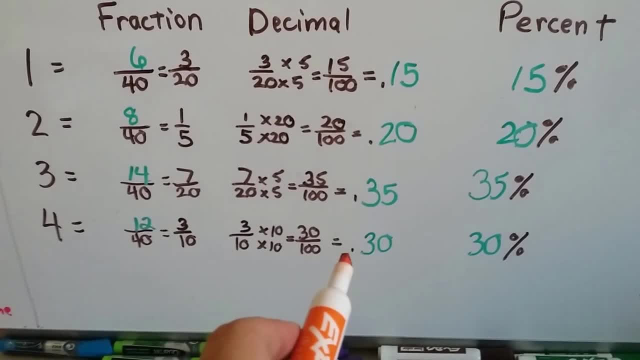 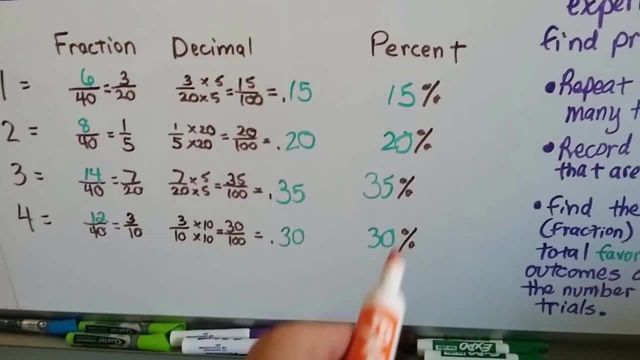 7 20ths becomes 0.35. And 3 tenths becomes 0.3, or 0.30,. okay, Then, as a percent, we just take away that decimal point and put the percentage sign in right. 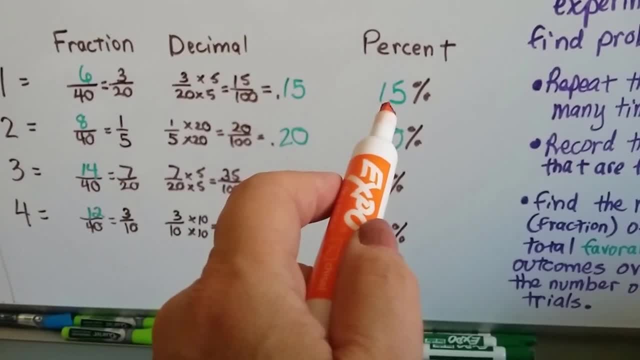 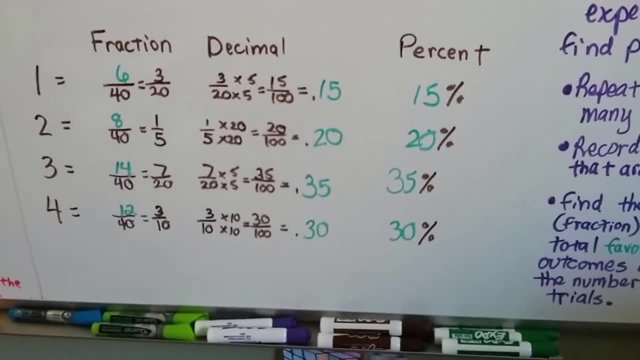 Because it means 15 hundredths, 15 parts of 100.. And that's what a percent is: 15 parts of 100.. So we've got 15%, 20%, 35% and 30%. okay, That wasn't that hard, was it? 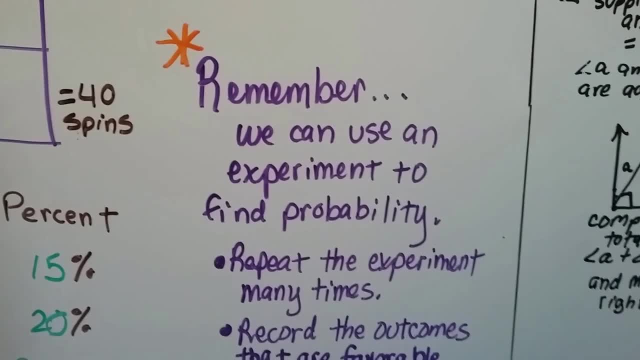 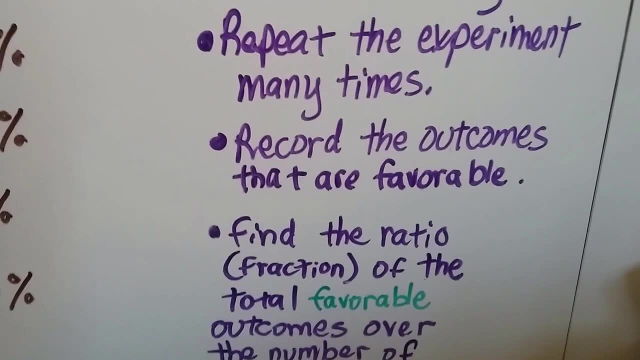 You can convert these. So here's what I want you to take away from this. I want you to remember that we can use an experiment to find probability. You repeat the experiment many times, You record the outcomes that are favorable. Then you find the ratio, the fraction of the total favorable outcomes.